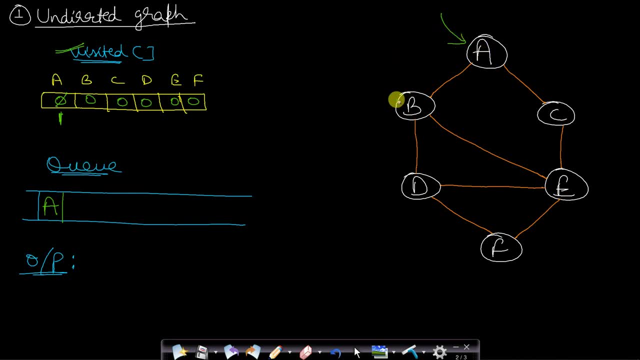 enqueuing this a into the queue. so the process goes like this: we first dequeue from the queue, so a is dequeued and our current element is a. now we will print the current element and then we will look at all the nodes which are adjacent to the current element and has not been visited. so 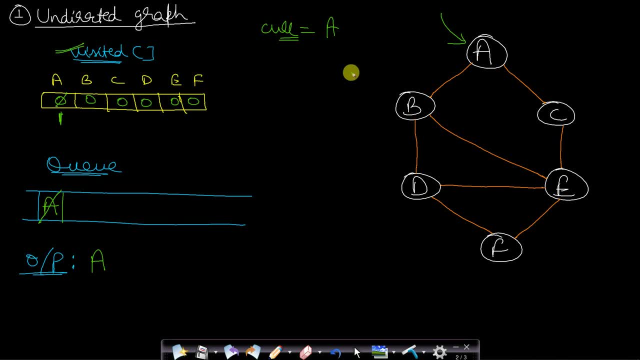 adjacent to a, r, b and c. both of them are not visited since in the visited array they have value 0, so we will push both of them. b will be pushed and the visited array value will become 1. c will be pushed and the visited array value will become 1. now a has been processed. 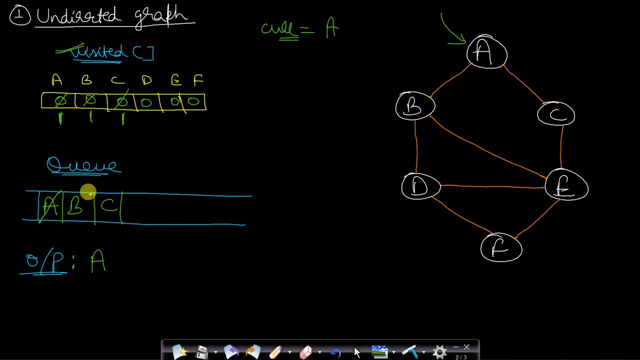 now. in the next time we will pop the next element, so b will be popped and our current element will now be b. so we are at b now. from b you can see that the adjacent or nodes are 3, a, e and d, but you can see that a has already been processed, since it's visited is 1. 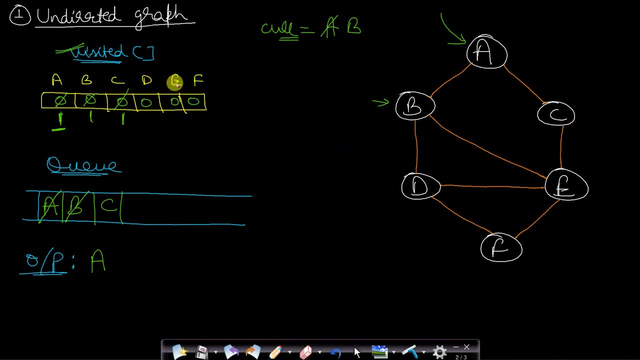 now e and d are adjacent and e and d value is 0 for the visited array. so we will add both e and d. so e will be added, d will be added and we will make the visited value equals to 1. that means they have been visited now, when we had popped it. actually we 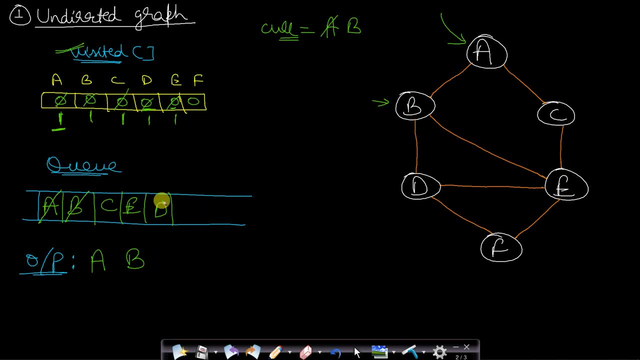 needed to print it as well, so this was prior to including the adjacent nodes. so now what we will do is we have added the nodes which are adjacent to node b, so this has been processed. now we will dequeue the next element, which is c, so our current element will now be c. so we will be at c now, since 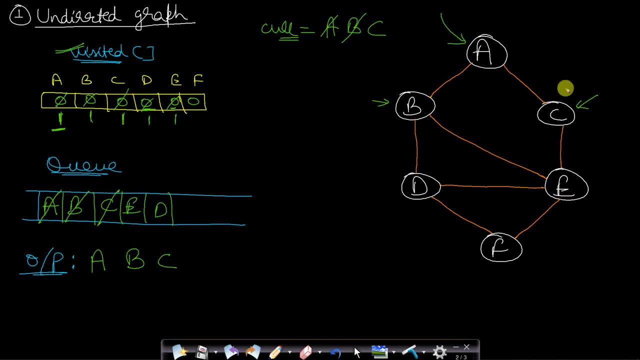 we have dequeued this c, we will print this c and then we will look at the adjacent nodes. now the nodes which are adjacent to c are a and e. both of them have been visited, since you can see that for a, value is 1 and for e value is 1. therefore, we assume that both of them have been added to. 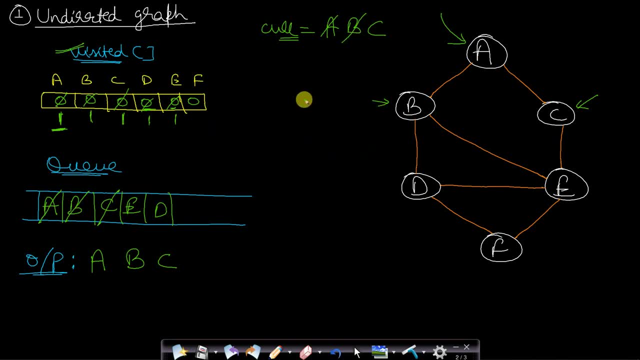 this queue. actually, in this bfs, we are assuming that whatever node has been added to the queue has been assumed to be visited, and so we will not add anything for this node. so this has been processed as well. now the next node which will be popped out is e, so our current 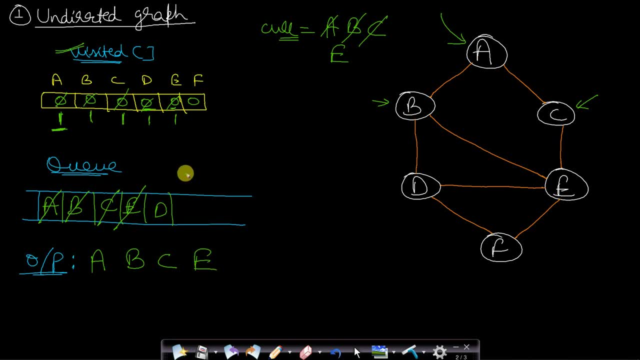 node is e, so we will print this e. and then we are at node e, so we will look at the adjacent nodes. adjacent to e, r, c, b, d, f. now we will check in the visited array which of them has not been visited. you can see that c, b and d have been visited, since their values are one, and f is not visited. 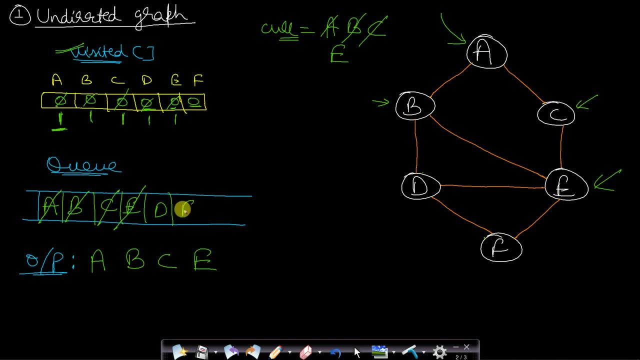 since its value is zero. therefore, we will just add f and we will make it visited now. e has been processed as well. now the next element is popped, which is d, so our current is d now. so we are at d currently. now we will print this d as well. now, from this d you can see that. 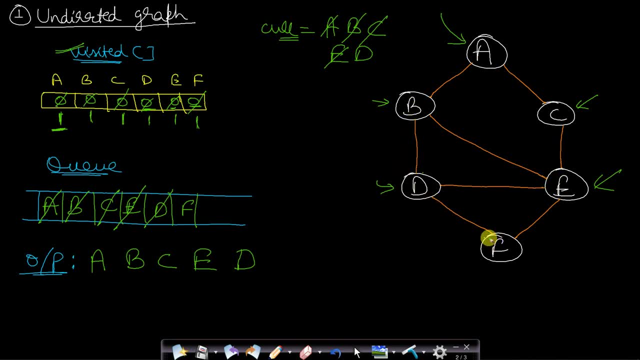 there are three nodes adjacent b, e and f. so you can see that all of them have been visited. since the entire visited array is one, all of them is having value one. so all of the nodes have been assumed to be visited. so we will not do anything for this d. now we will pop the next element, f. we will print this f. 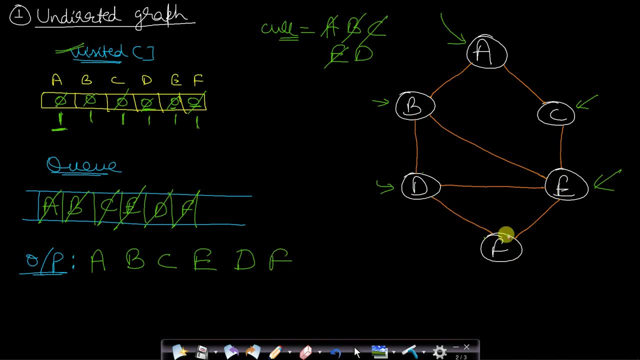 and then we will look at the adjacent nodes, which are d and e. they have been visited as well, since the value for d is one and for e is also one, so they have been visited. so we won't add them to q. so this has already been processed. now, now the q has become empty and this signifies that we have. 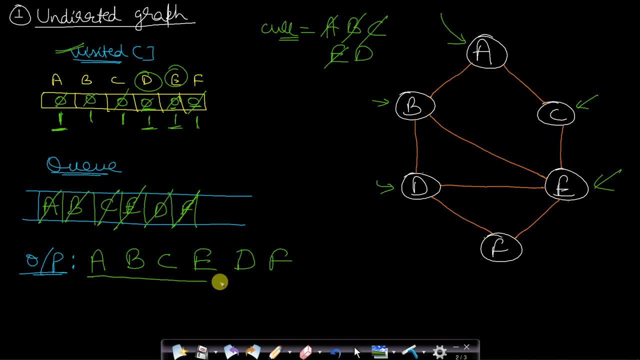 in this graph and whatever has been printed, that is a sequence of our traversal, is the breadth first search or the breadth first traversal, which is bfs or bft. now you should notice one thing, which is that we have made choices like: from a we were adding b first and then c. you can see that. 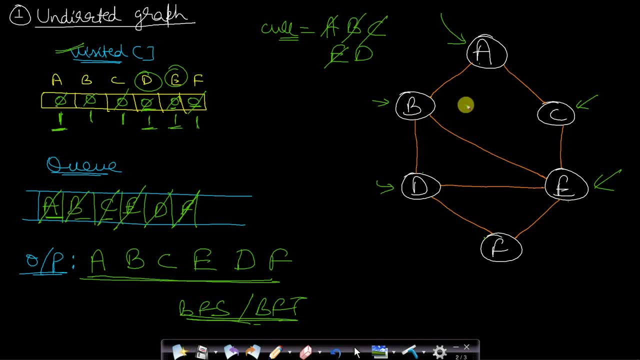 in the queue we have written a, b and c, because from a we added b and then c. but we could have followed another order. we could have added c first and then b, so the entire sequence would have changed. so there can be more than one sequences for a given graph, for bfs or bft. 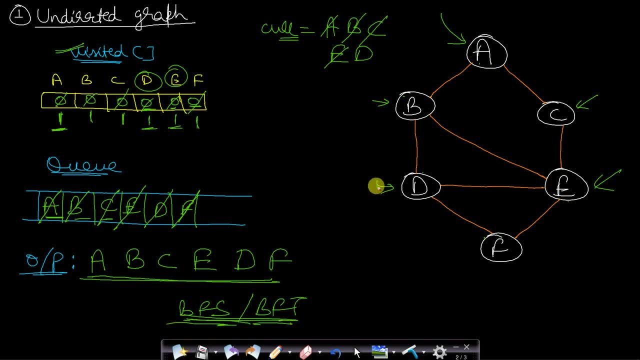 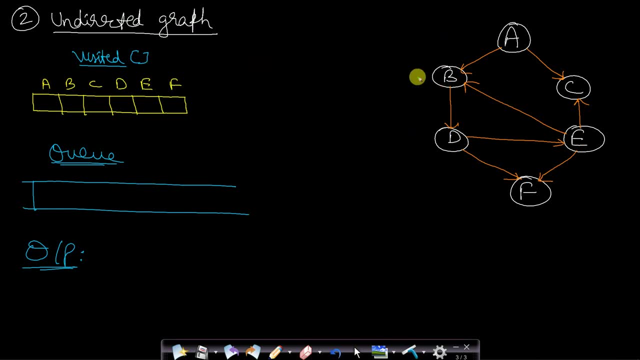 so this you should keep in mind. so let us look at the directed graph case. i have already made a directed graph which is similar to our previous graph. in this case as well, we need the visited array to keep track of the visited nodes, and then we need a queue. 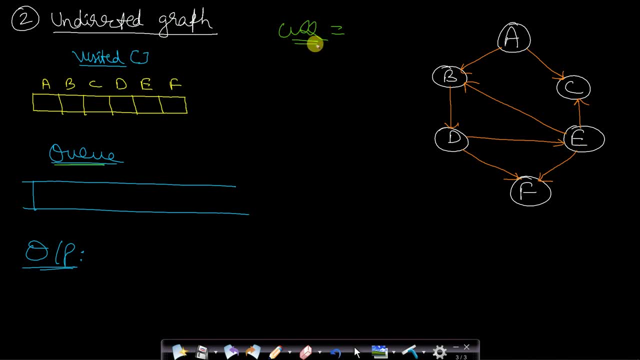 you. we will take a current pointer, okay, which will be null initially. and then let's say we are starting from this node a and, by the way, before starting, none of the nodes will be visited, and so all zeros will be initialized to the visited array for all the nodes. now we will be starting at a. let's say: 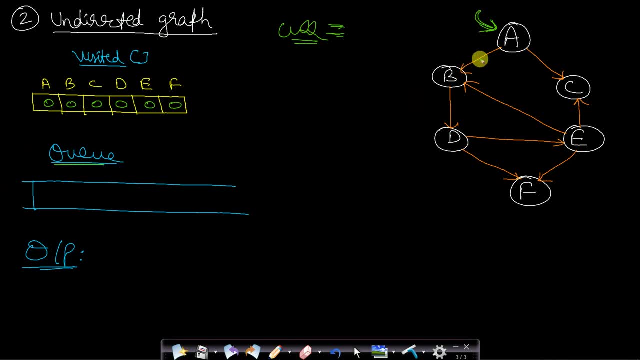 we will be starting at a. so what we will do is, before starting, we will push the first element and we will make it a null, and then we will take a current pointer, which will be null initially, and we will make it visited as one. now, how do we start? we will start from this a. we will dequeue the. 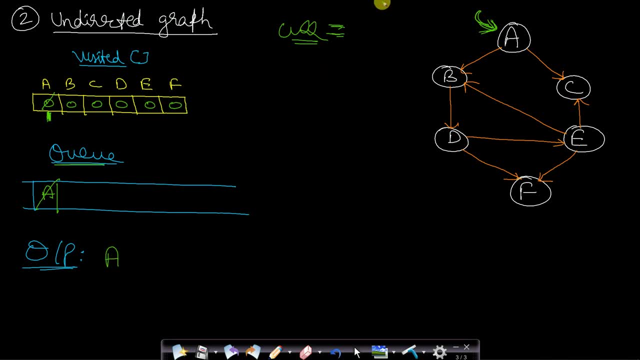 element from the queue. we will print it. this is our current element a. now from a we will look at the adjacent nodes. adjacent node that is outgoing edge from a is going to b and another edge is going to c. so there are two adjacent nodes. so what we will do is we will add. let's say we add b first. 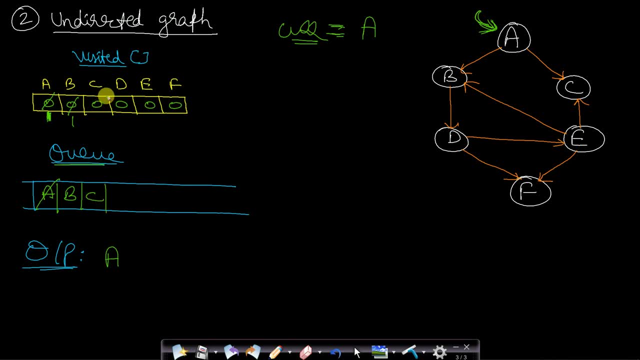 we make it visited, we add c next and we make it visited. now. both of them have been added. so a has been processed. now we will dequeue the next element. so when we dequeue b comes out, we will print this b. our current element is b now. now we are at b. from this b you can see that there is. 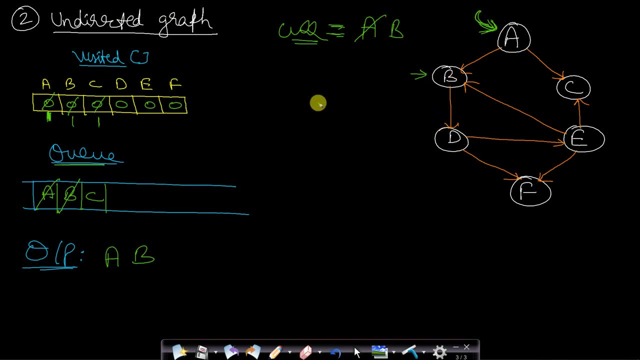 only one outgoing edge, which is to d. we will check this in our visited array. d has never been visited. value is 0. therefore, what we will do is we will make it visited and we will add d to the queue. now this node b has been processed, so we will dequeue the next element, which is c. so c will be dequeued. 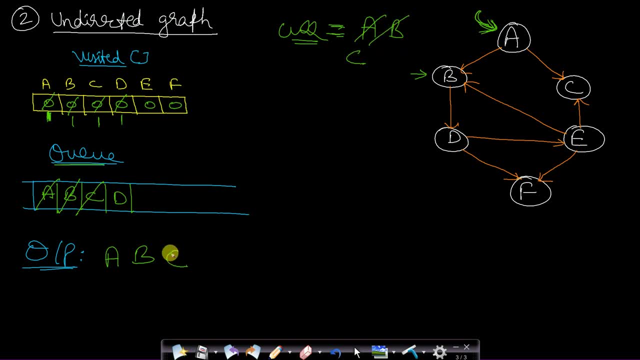 our current element will be c. we will print c. now we are at c, so from this c you can see that there is no outgoing edge. so we will not add anything. so this node has been assumed to be processed now. so we will dequeue the next element, which is d. d will be dequeued. we will output d, our current. 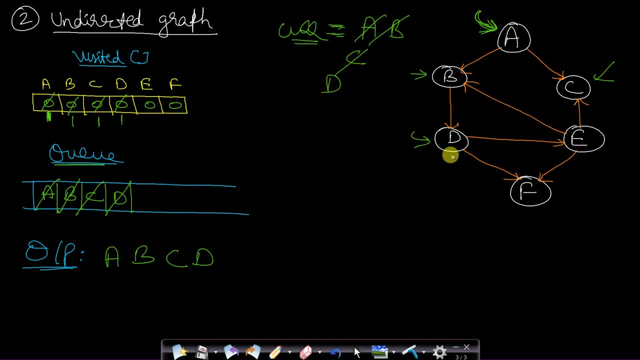 element will be d now and we will go to d. from this d you can see that there are two outgoing edges to e and f. so let's say we want to go to e first. so we will check in the visited array and there the value is 0, we make it 1, we add it to q. now for the next node, which is f, we check it in. 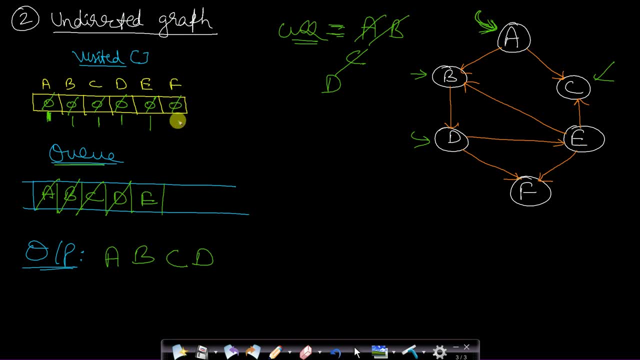 the visited array and it is 0, that means it has not been visited. we will make it one. we will add it to q. now we have processed this node d. now what we will do is we will dequeue the next element, which is e. so our current element is now e. we will output e and we are at e from this e. you can see. 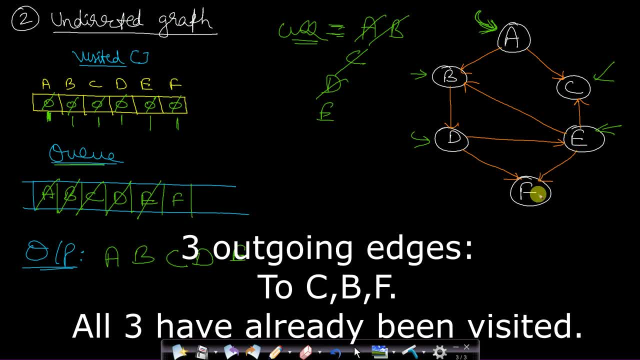 that there are two outgoing edges. one is going to be another, one is going to f, but both of them have already been visited, since you can see that in the visited array for b and f there are values 1, so both of them are assumed to be visited. therefore, this is also 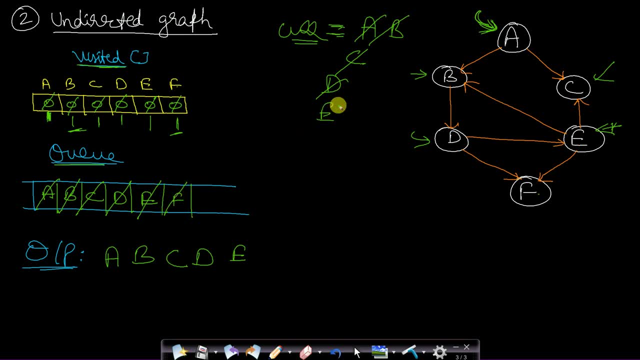 processed. now we will dequeue the next element, f. our current element is now f. we will print f. we will go to f from f. there is no outgoing edge, so this is also processed. now the sequence which we got is the BFS or the BFT of the given graph. now, as I said earlier, there can be many possible. 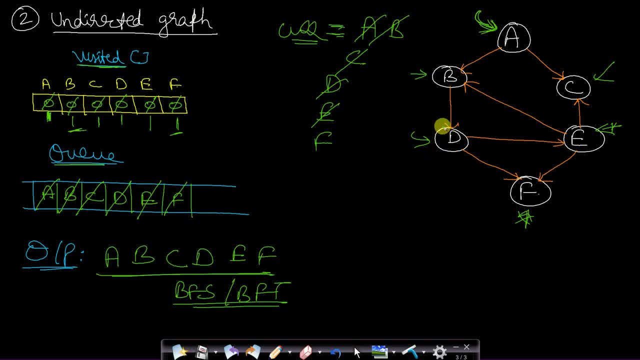 BFS or BFT for a single graph and that depends on the choices which we have made, like I said in the previous graph, So you should try out different, different sequences in order to understand better. Now let us look at the code for this: BFS or BFT. 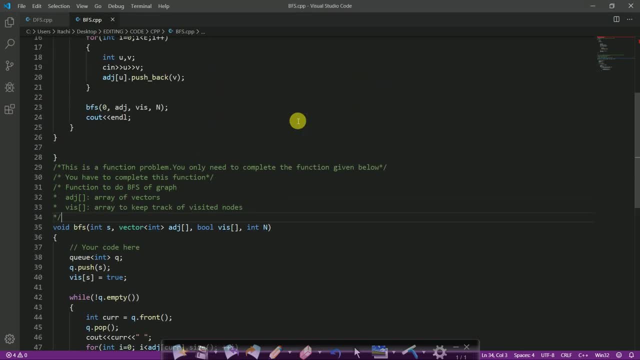 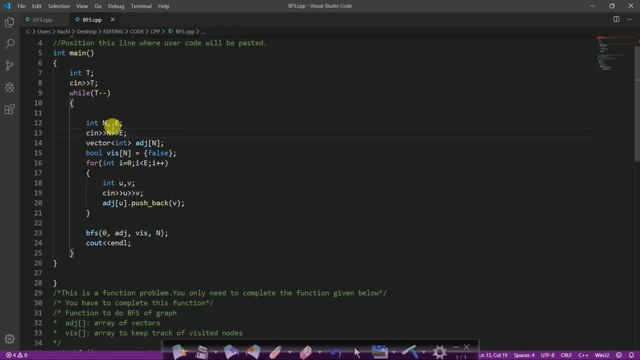 So this is the code which I have written to implement BFS or BFT. First is T, which is showing the number of test cases, Then there is N, which is showing the number of vertices, and E is showing the number of edges. Now we have taken an adjacency list and we have implemented it by using vector of vectors. 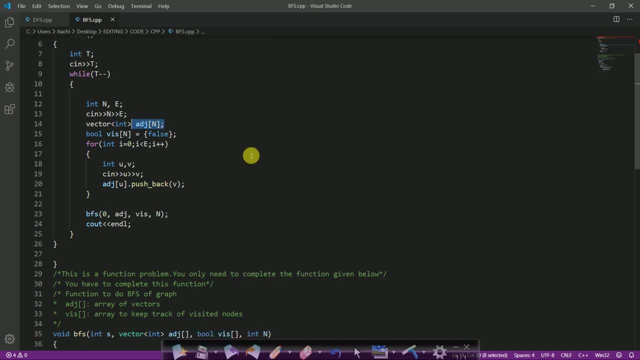 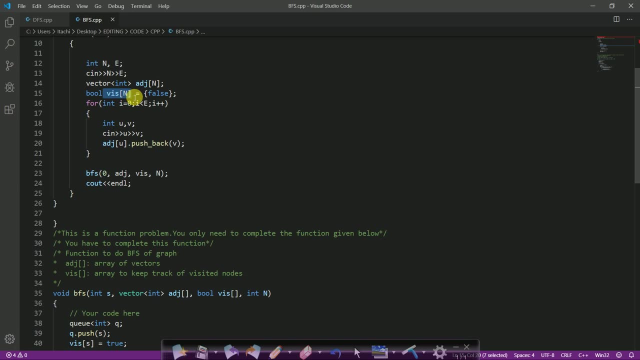 So if you have any type of doubt in adjacency list then you should watch my video on representation of graph. So I have taken a visited array and initially I have initialized all the N elements to false. Then I have taken input of all All the E edges and I will just push them in the vector of vectors. 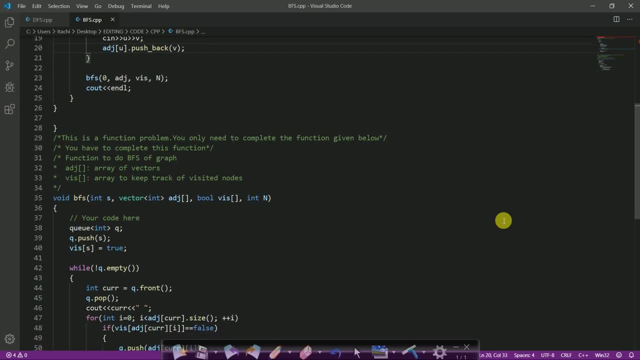 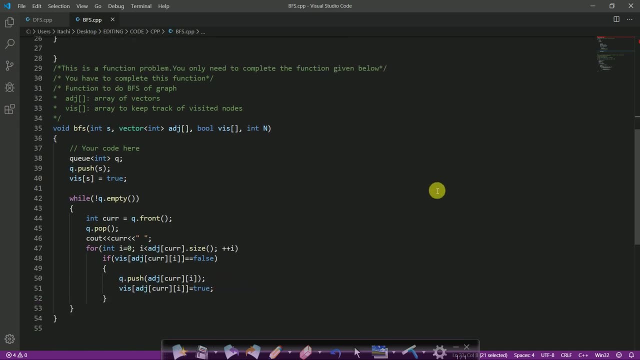 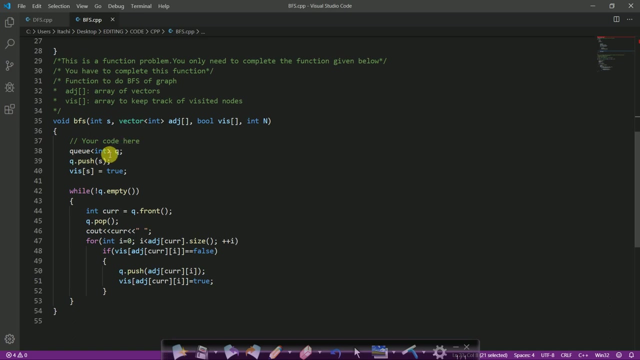 So, after preparing the data, after taking all the inputs, I have called BFS, BFS is called and the starting node is taken as zero. So this is the entire code for the BFS. This is a very simple code and it just works as I have explained in the theory part. 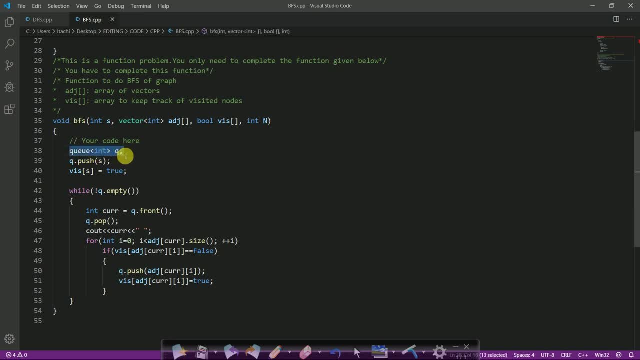 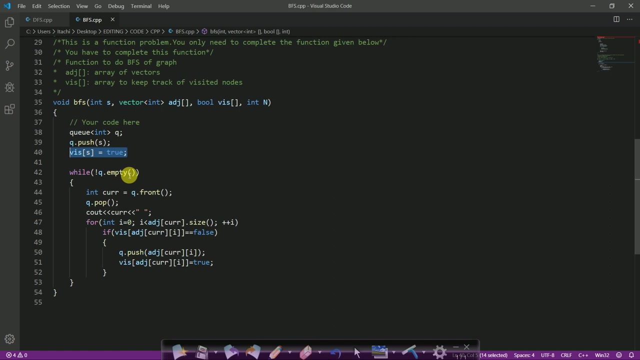 So first we will take a queue. This is an iterative process. First we take the queue, We will push the code, We will push the starting point in the queue and then we will make the visited of the starting point equals to true. Now we will run this loop in line number 42 till the queue is not empty. 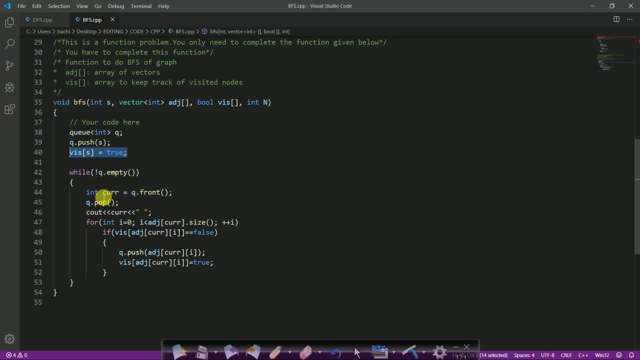 So until the queue becomes empty, we will run it. Now what we will do is we will take the first element out from the queue, We will pop this first element and then we will print it, like we did in the theory, and then after that. 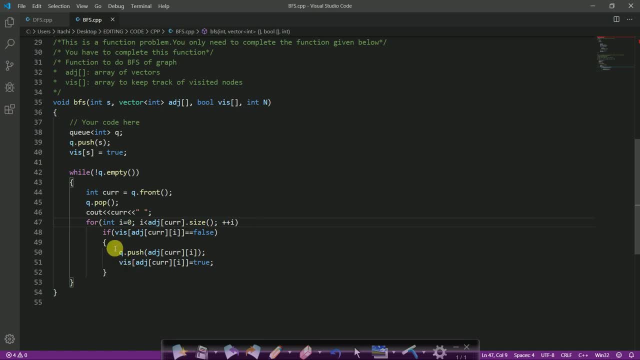 We will visit all the adjacent edges. So we will check. if the adjacent edge is not visited, Then we will push the adjacent node in the queue and then we will mark it visited, like I have already explained, And then again in the next loop, again the next element will be popped out.